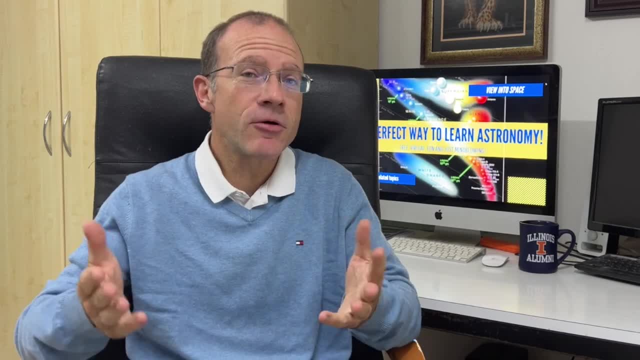 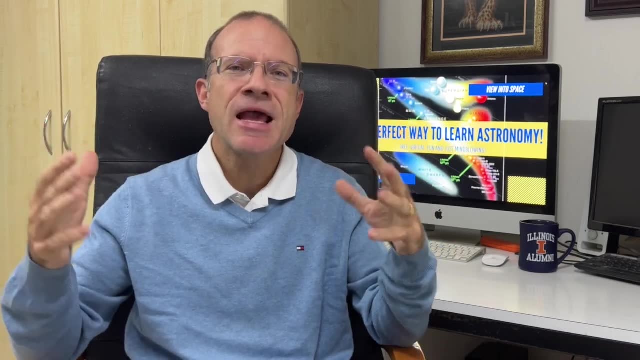 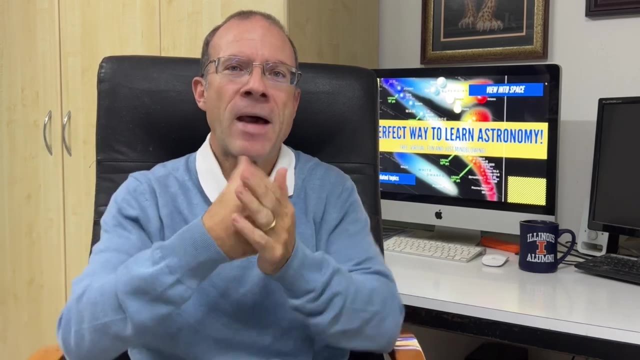 Now imagine the same situation, the same question And you go like: oh, planetary nebula. That's actually when a rare giant in its late stage is expanding and its glowing shell is ejecting ionized gas which causes this emission. nebula, Bam, that's impressive. 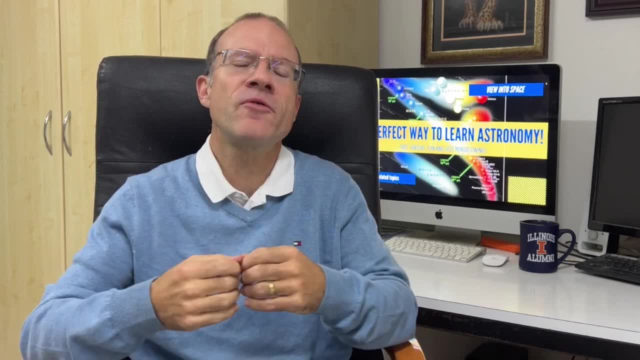 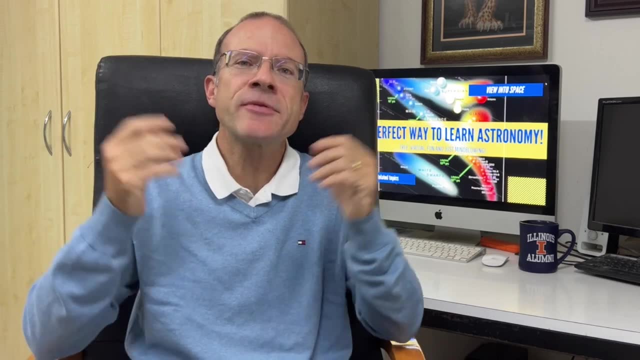 And, by the way, that's also quite useful to know for yourself. My point is: when I started this hobby, I couldn't see enough. I couldn't capture enough of what I saw, So I'm going to show you how to do it. 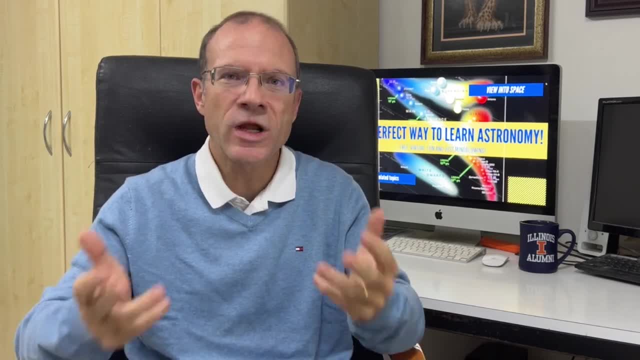 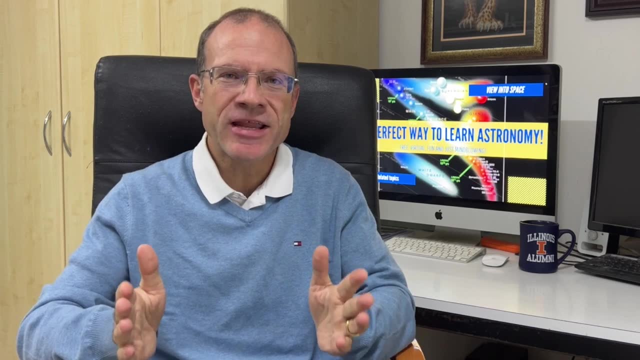 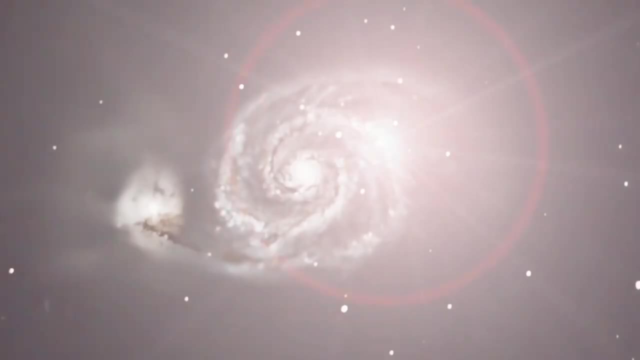 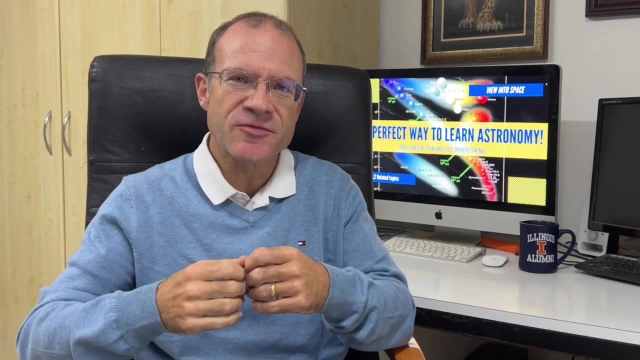 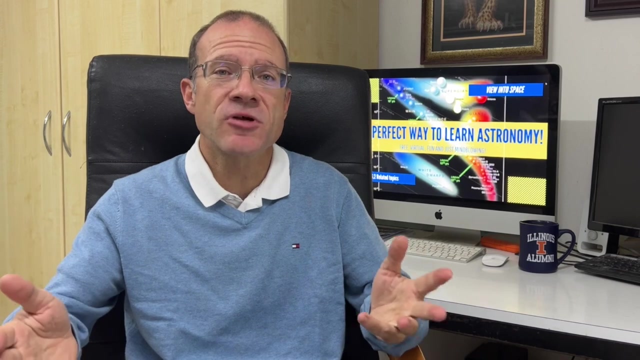 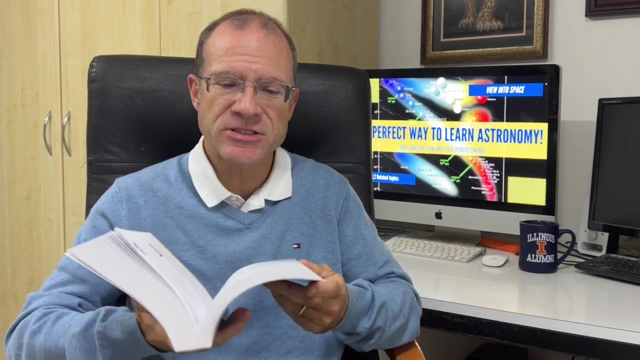 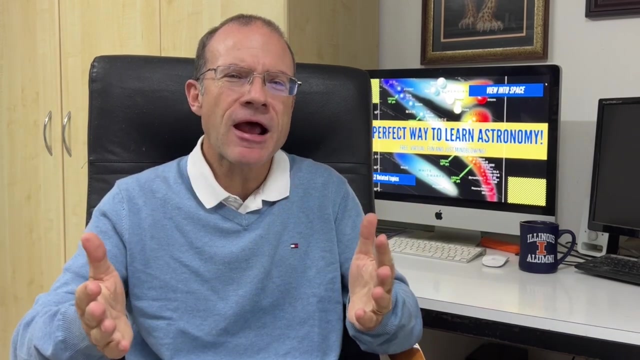 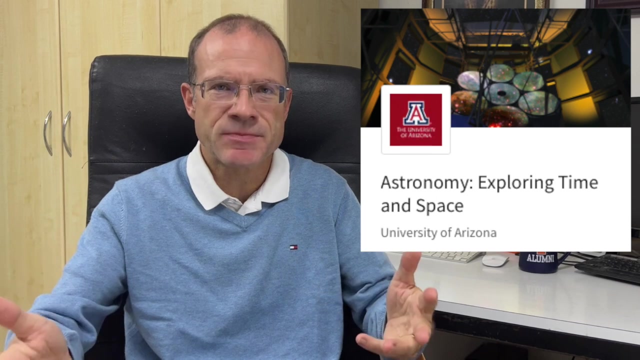 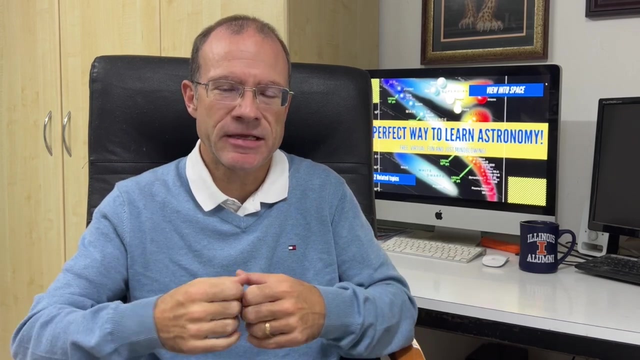 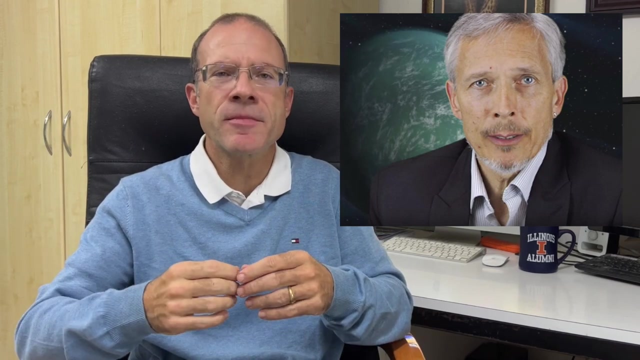 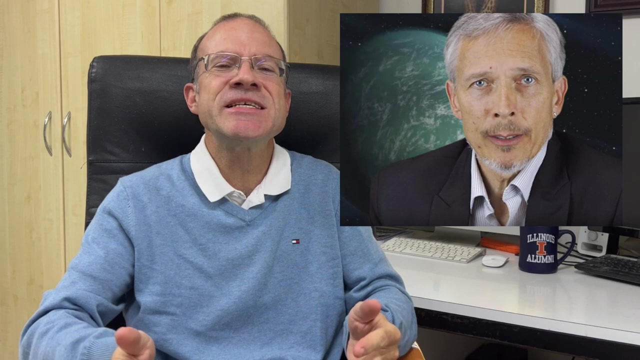 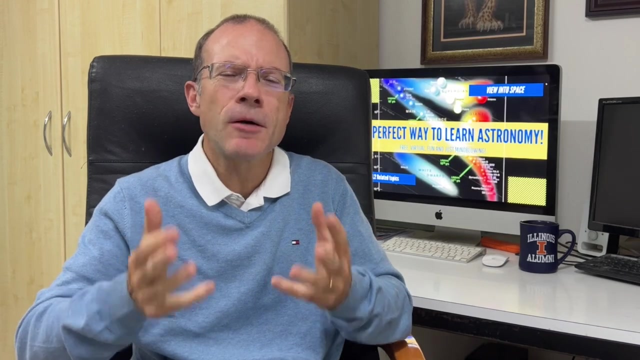 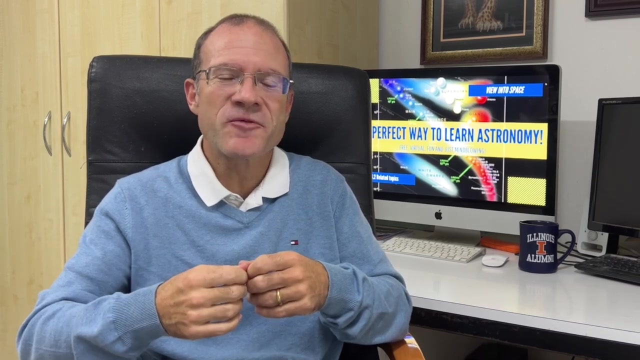 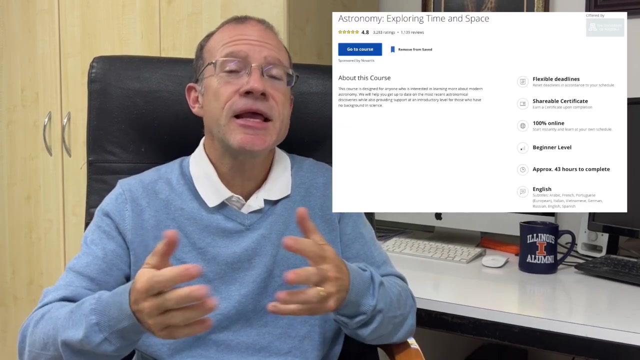 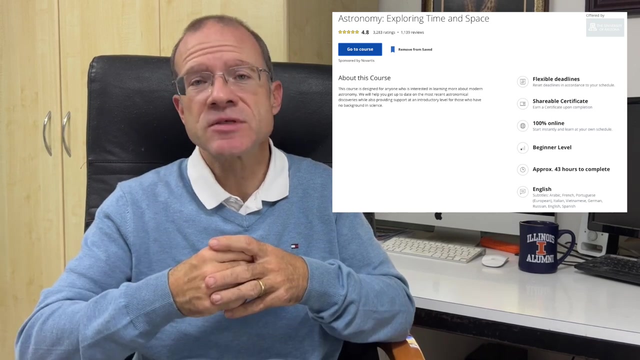 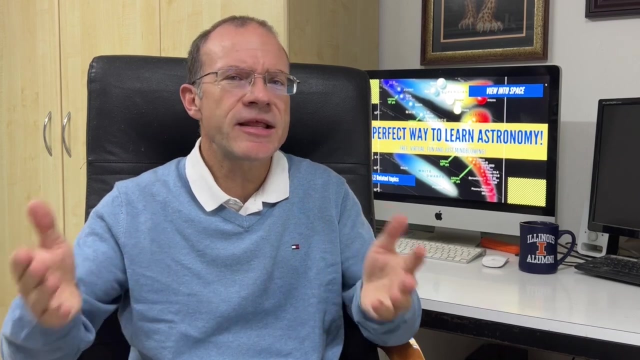 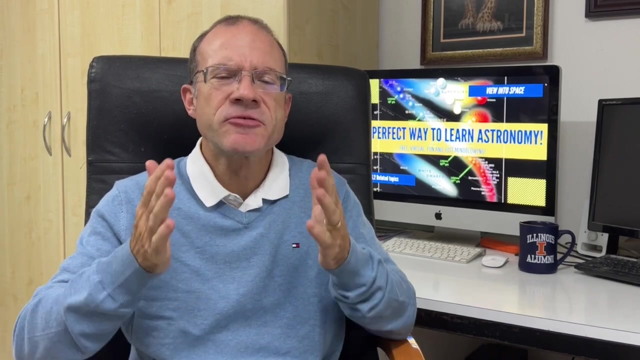 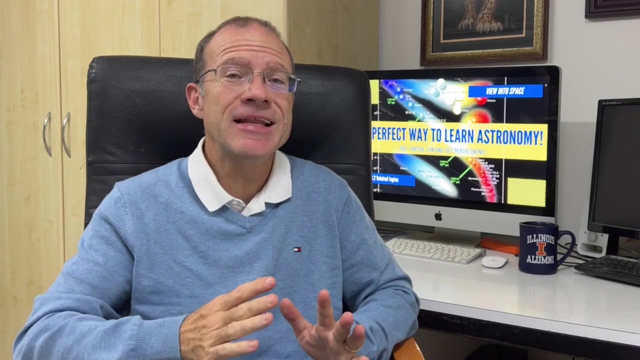 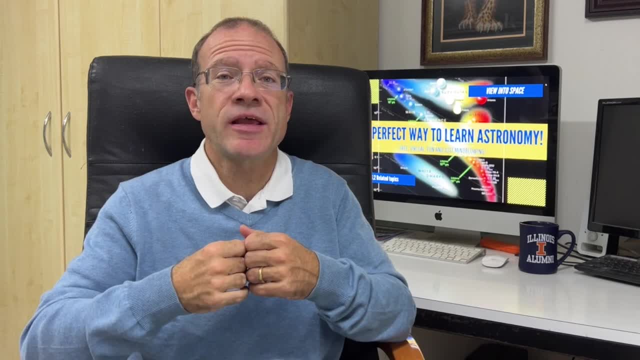 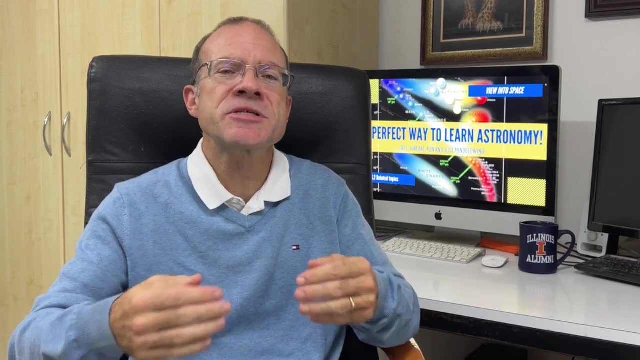 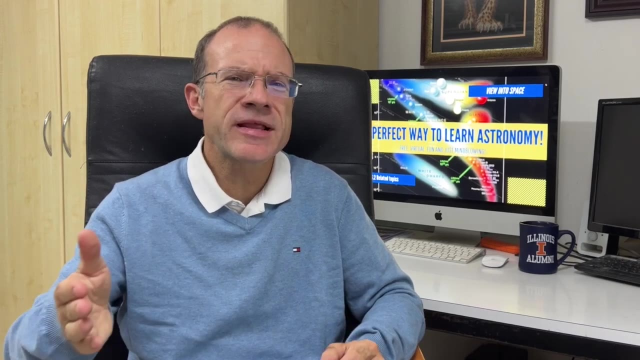 So, given that this is such a fast-moving science, certain things are already a little bit outdated or just not 100% up to date, But the coolest part is that Professor Impey does about, I think, two or three times a month, live sessions. 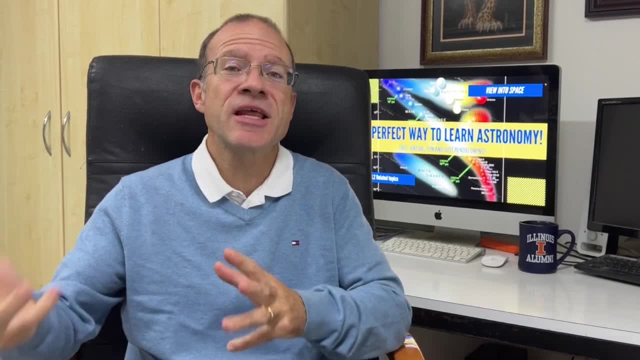 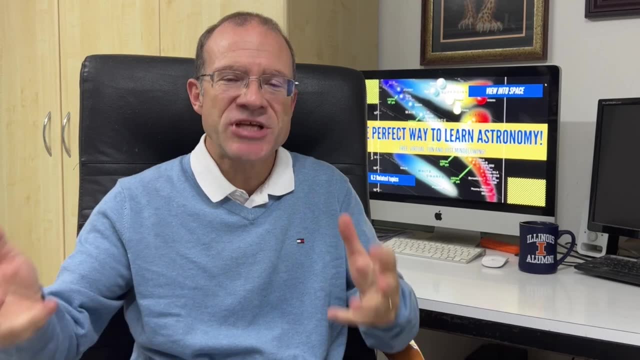 in the tent and you can ask questions. So there, actually, he fills all that in. that actually also happened in the last 10 years. So let's have a look at the 10 chapters of this course that you have an idea what is covered. 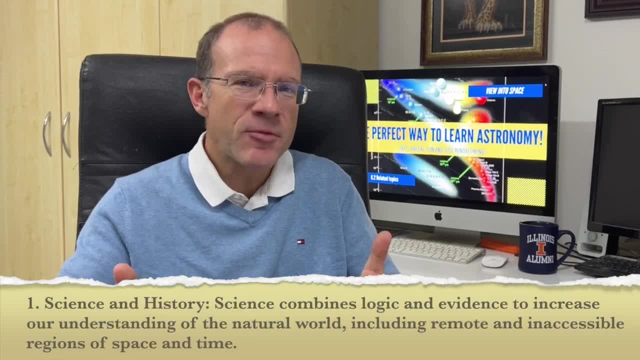 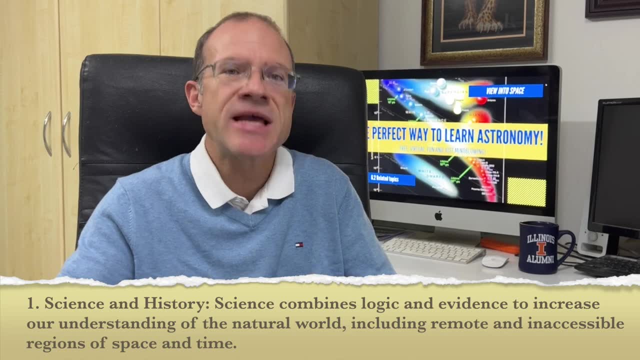 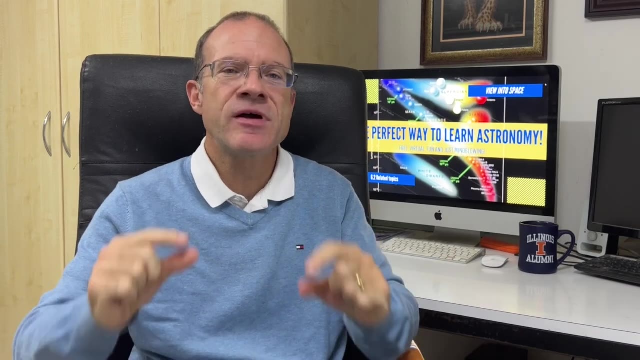 Chapter one is called Science and History, And Professor Impey really starts with giving you an understanding what science is, because everything is based on science. So while this might seem a little bit far-fetched for astronomy, it gives you a very good foundation, also nomenclature-wise. 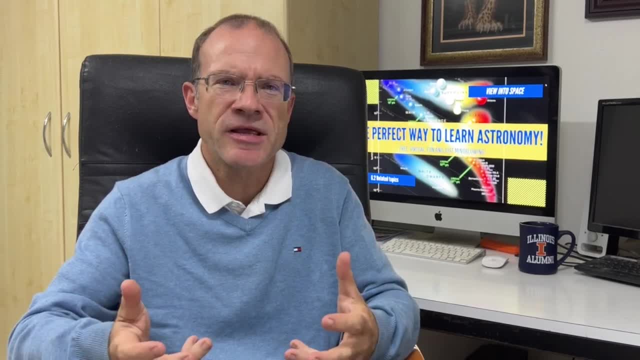 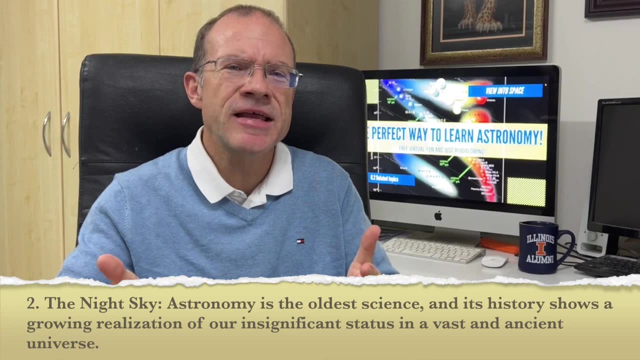 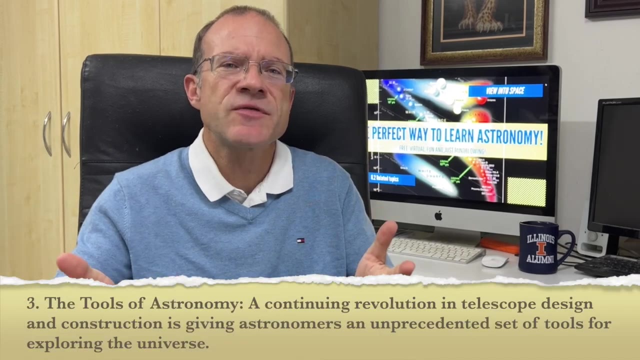 He also covers here the roots of astronomy, how ancient people used the stars for their daily lives. In chapter two, the night sky, he goes on with the history, with the discovery of the telescope and so on. And then in chapter three, the tools of astronomy, he really starts discussing about the different types. 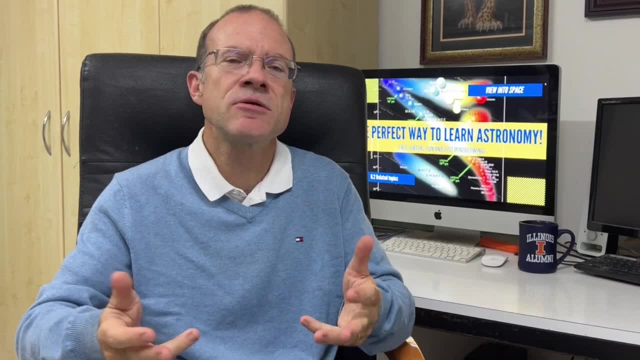 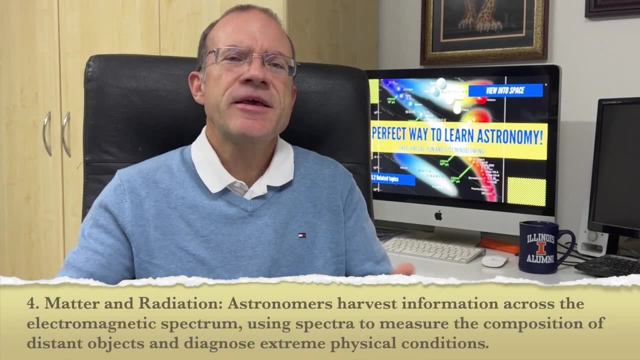 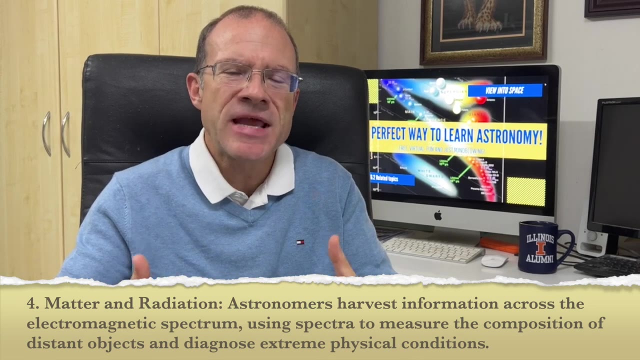 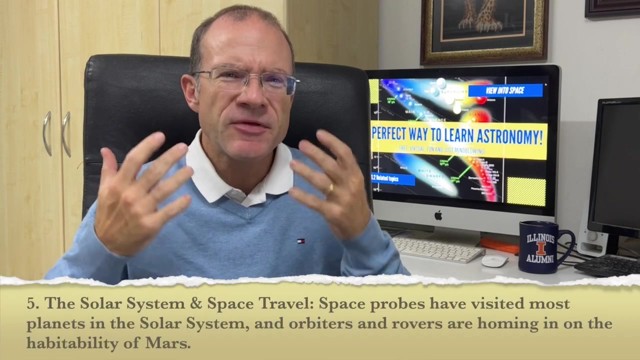 of astronomy telescopes and radio telescopes and so on that are actually available to us to discover the skies. In chapter 4 he goes again to the foundation and discusses matter antimatter radiation, just the basics with which we actually can measure what is happening in space. In chapter 5 he discusses the solar system. 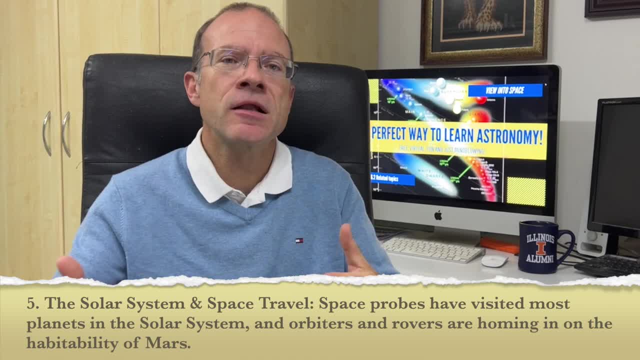 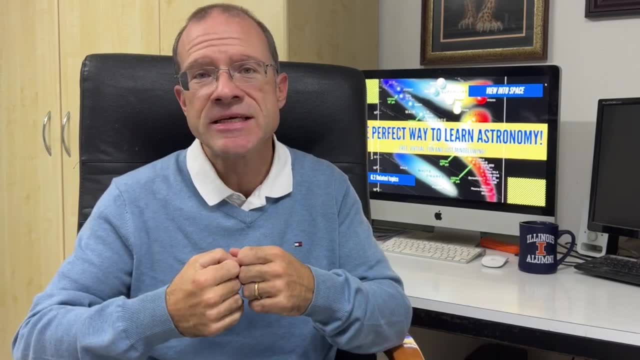 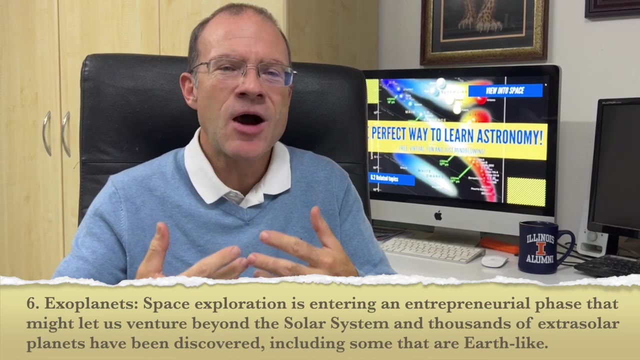 and space travel, what mankind has already done, exploring the Moon, Mars, Venus and so on, so all the space probes we have already sent to space. In chapter 6 he has a look at exoplanets: what they are, how we try to discover. 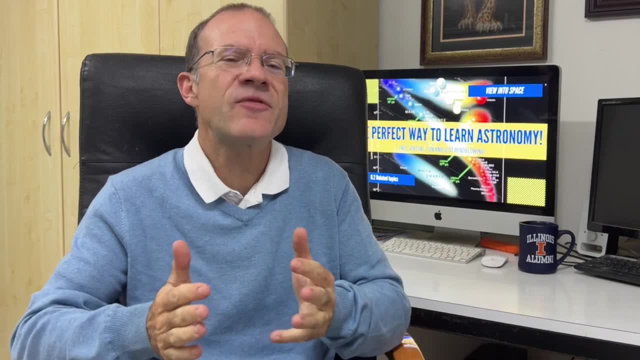 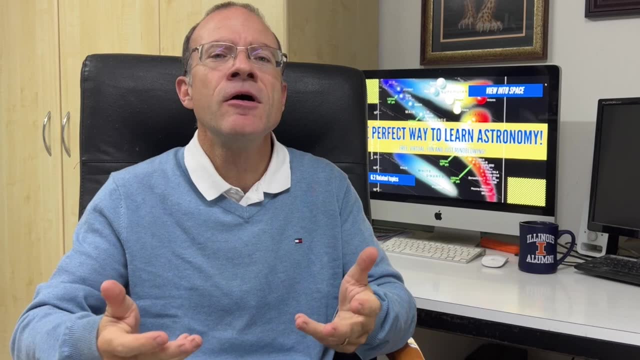 them, what meanings they have. quite fascinating, this chapter, And I think, when we go now into astrophotography, chapters 7 and 8 are the most relevant to us. Chapter 7 is about the star birth and death which it also 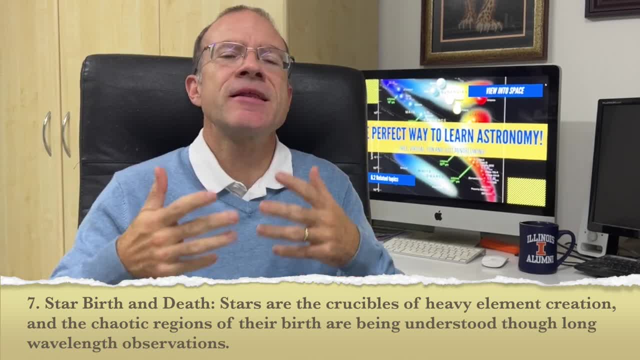 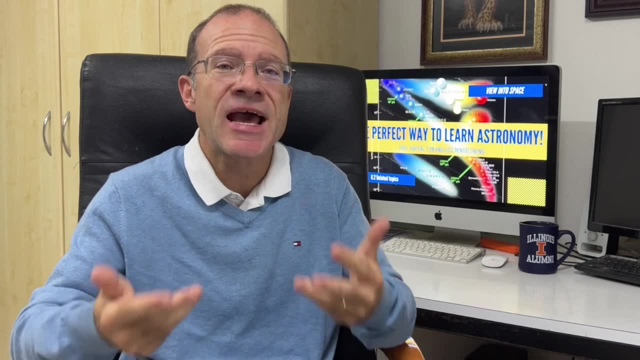 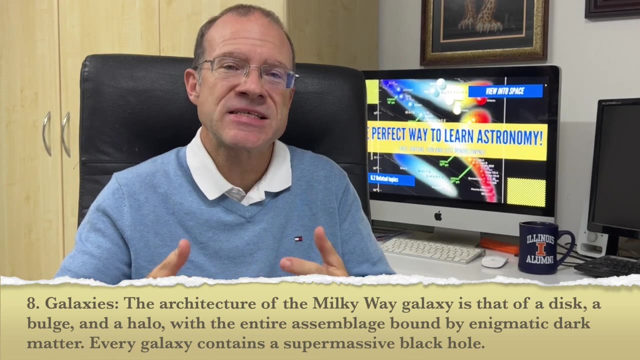 leads to all the nebulas, And so here we really get an understanding how the different types of nebulas get generated and what's actually happening within them. In chapter 8 he covers the galaxies, and also here I found that absolutely fascinating that, based on the shape, on how galaxies look like, we can actually